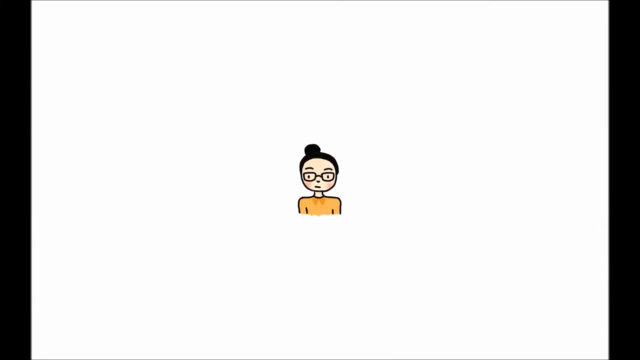 So in this example, the solution is 3, 2.. But wait, how did you just figure that out? Well, this brings us to our lesson. There are three ways to solve a linear system: Graphing, substitution and elimination. I'll turn this over to Maya and she'll show you how to solve linear systems by graphing. 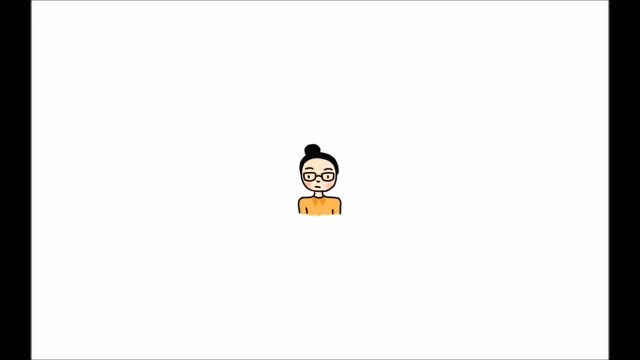 Hey, it's Maya and I'm here to teach you how to solve linear systems by graphing. Let's use the two equations from before as an example, In case you forgot. the equations are: x plus 2y equals 7, and 3x minus 2y equals 5.. 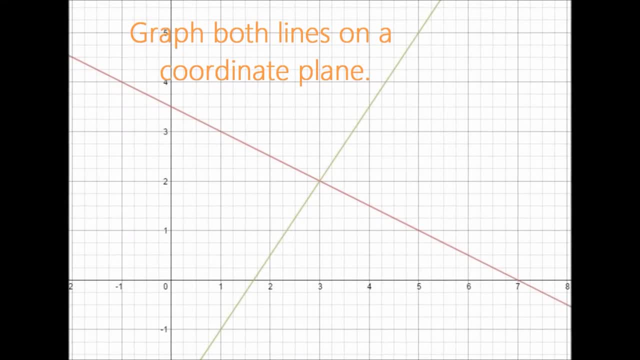 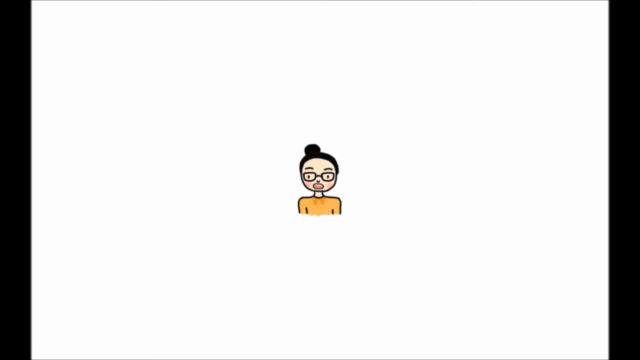 First you graph both lines on a coordinate plane. You can do this by finding the x- and y-intercept or changing both equations to slope-intercept-form and slope-intercept-form and then graphing them. Then all you have to do is find the point. 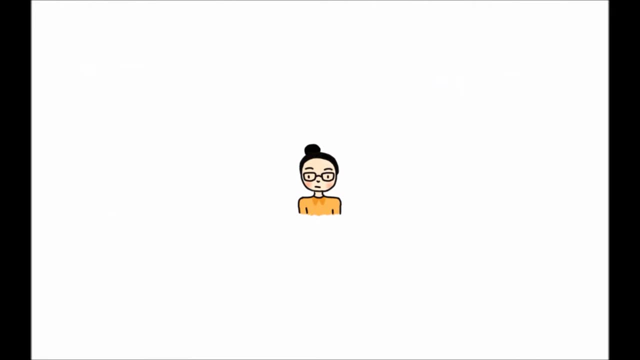 where your lines intersect. That's it. that's your solution. You may need to estimate the ordered pairs other times when using this method, and be sure to check your solutions a couple of times as well. This is usually the least preferred method of solving systems of linear equations. 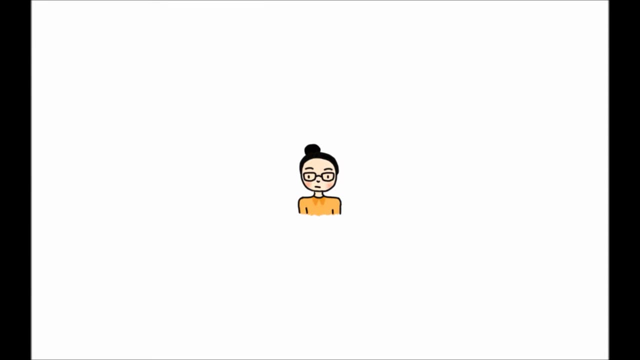 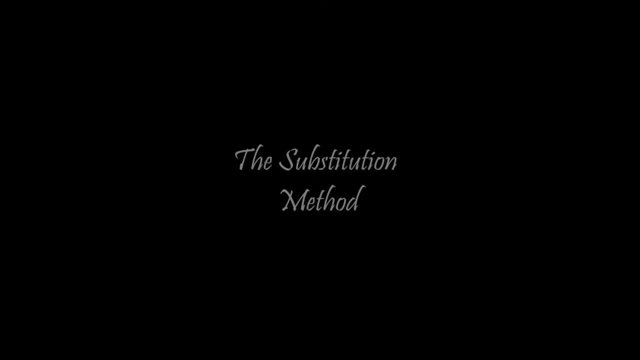 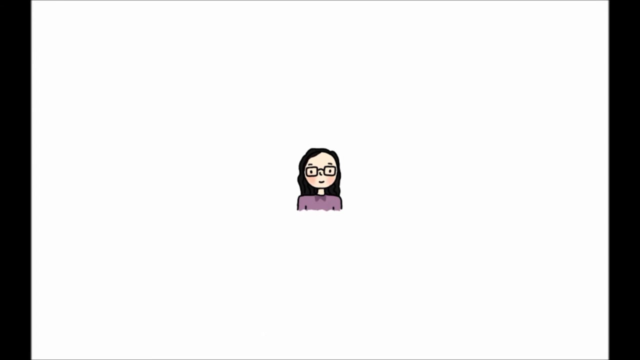 because it takes the longest, but if it's your cup of tea, then go for it. The next method to solving linear systems is substitution with Abby and Jasmine- Oh wait, that's me. Substitution is one of the more popular methods of solving linear systems. 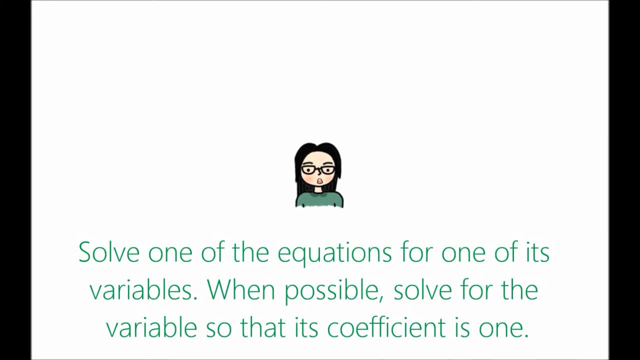 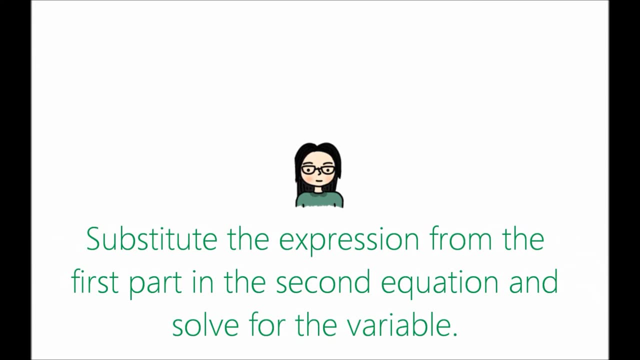 Let's see if it's the one for you. First, solve one of the equations for one of its variables. When possible, solve for the variable so that its coefficient is one. Second, substitute the expression from the first part in the second equation and solve for the variable. 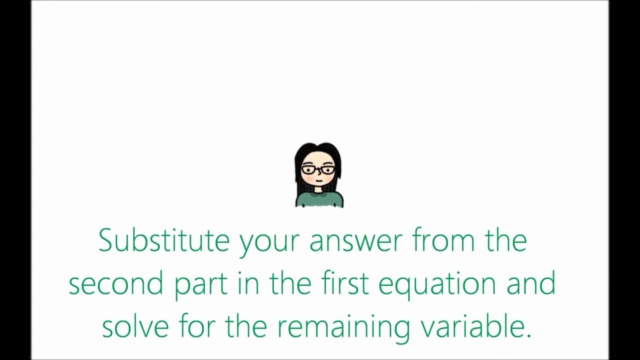 Third, substitute your answer from the second part in the first equation and solve for the remaining variable. It's that easy. Still don't get it? Let's try an example. Let's solve for the following equations: 4x plus 6y equals 4, and x minus 2y equals negative 6.. 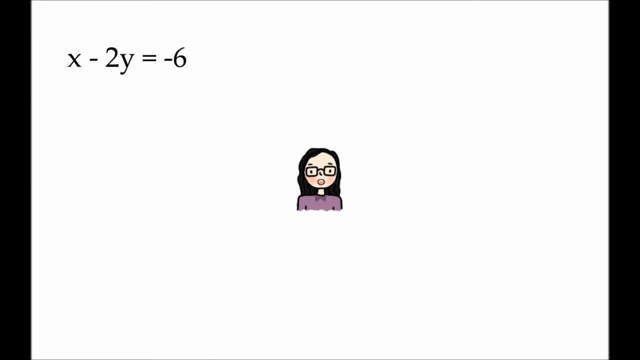 Step one: since x minus 2y equals negative, 6 has a variable with a coefficient of 1, let's solve for x. Step two: now substitute the rewritten equation- x equals 2y minus 6, for x in the other equation. 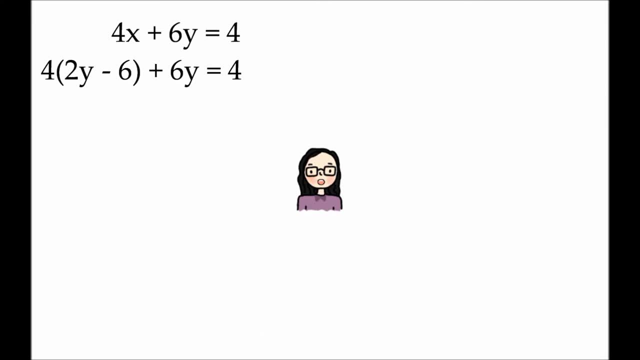 Step three: Solve the variable by solving for y in the new equation 4, parentheses: 2y minus 6 plus 6y equals 4.. Step four: Substitute the y variable in the rewritten equation from before x equals 2y minus 6, with y equals 2.. 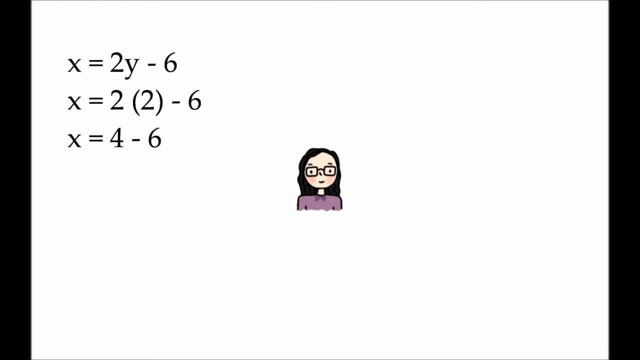 Step five, Finally, to isolate the variable solve for x. in the new equation, x equals 2 times 2 minus 6.. So there you go. The answer to this system of linear equations, as you saw before, is negative 2, 2.. 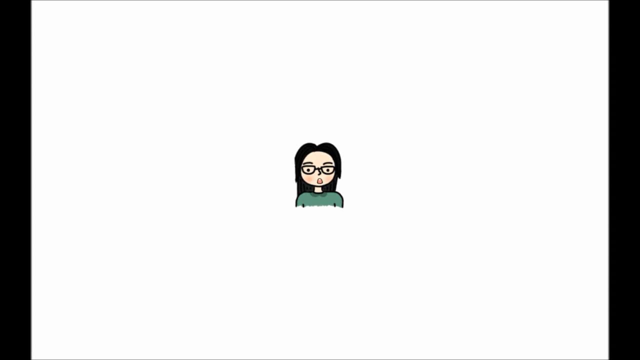 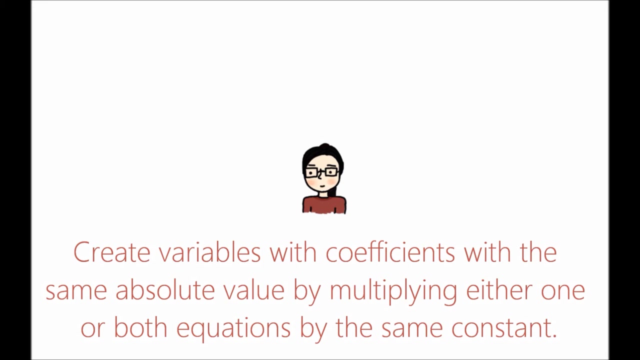 2. Now on to learning how to solve systems using the elimination method with Kaylin and Jenny. To solve linear systems with elimination, you first have to create variables with coefficients with the same absolute value by multiplying either one or both equations by the same constant. 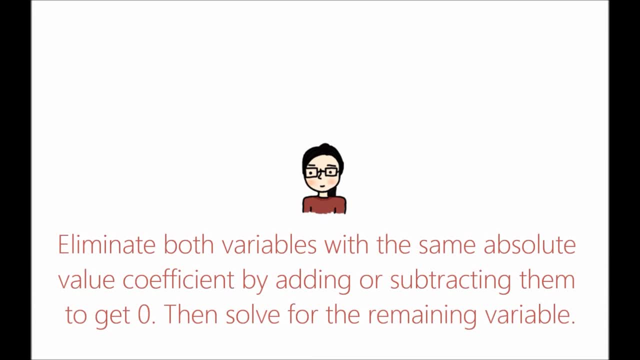 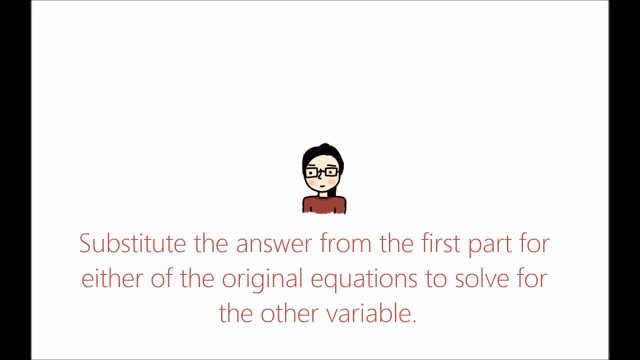 Once you have done that, you may eliminate both variables with the same absolute value coefficient by adding or subtracting them to get 0. Then solve for the remaining variable. Substitute the answer from the first part, 4x. Now you have to solve for either of the original equations. 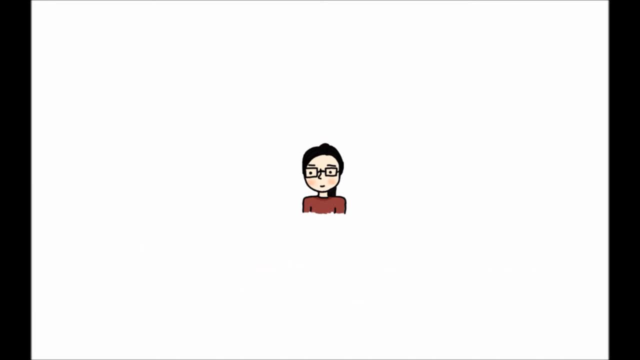 to solve for the other variable. Solve for the remaining variable to get your final answer. Let's solve the equations: 10x minus 8y equals 4, and negative 5x plus 3y equals negative 9, using elimination Step one. 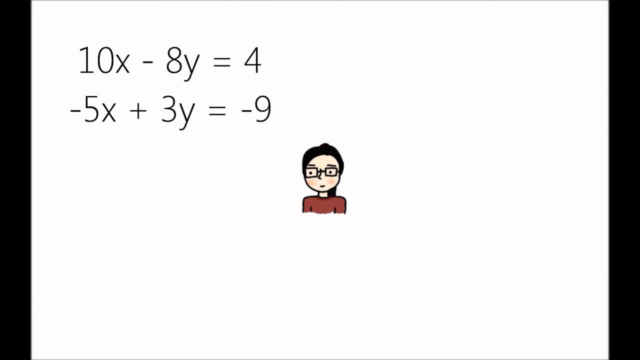 Write out the two equations one on top of the other, so that the like variables are lined up. Step two Then: multiply both or one equation by a constant, so that the same variable in both equations has the same coefficient, In this case the variable x in both equations. 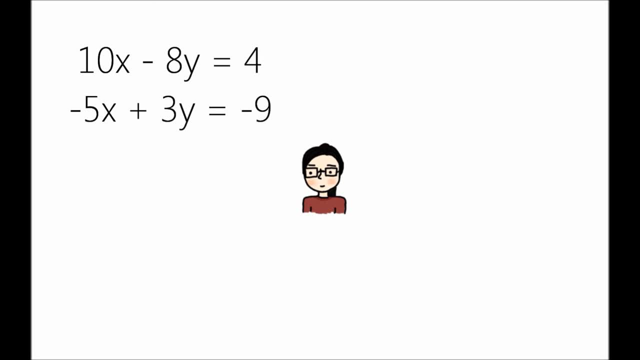 have coefficients that can be easily eliminated, because 5 is a factor of 10.. Step four: Multiply the equation negative 5x plus 3y equals negative 9 by negative 2 to get 10x minus 6y equals 18.. 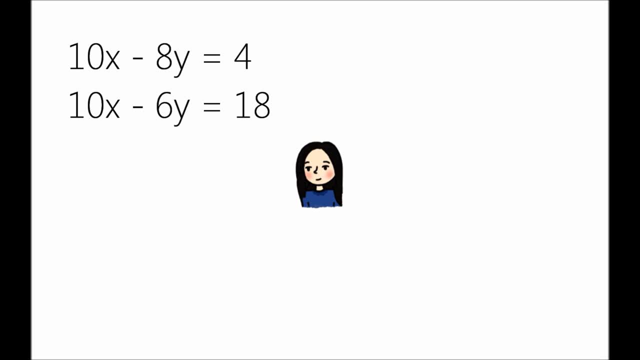 Notice that both equations now have the same term 10x. Step five: In order to eliminate the 10x from both equations, so that you can solve for y, subtract the equation 10x minus 6y equals 18 from 10x minus 8y equals 4,.